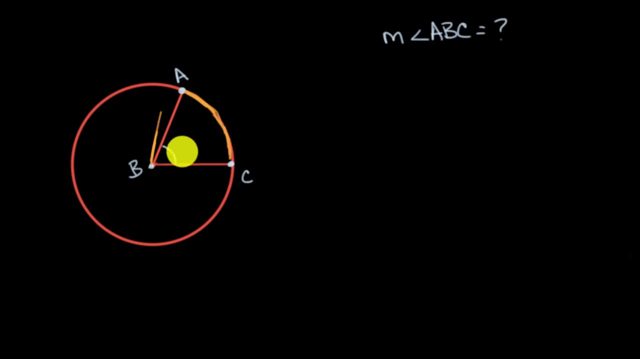 if it looks something like that, then the arc length would be larger. So should we define the measure of an angle like this as being equal to the length of the arc that it subtends? Is this a good measure? Well, some of you might immediately see a problem with that. 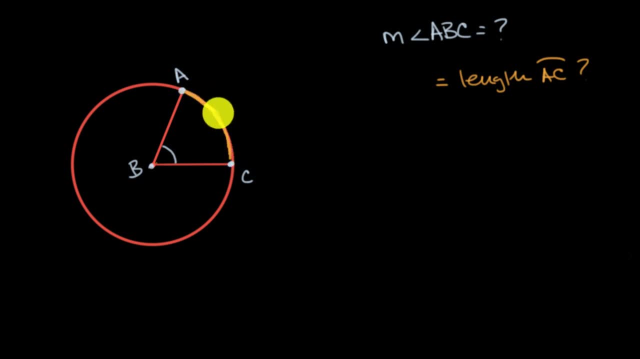 because this length, the length of the arc that is subtended, is not just dependent on the angle, the measure of the angle. It also depends on how big of a circle you're dealing with. If the radius is larger, then you're gonna have a larger arc length. for example, 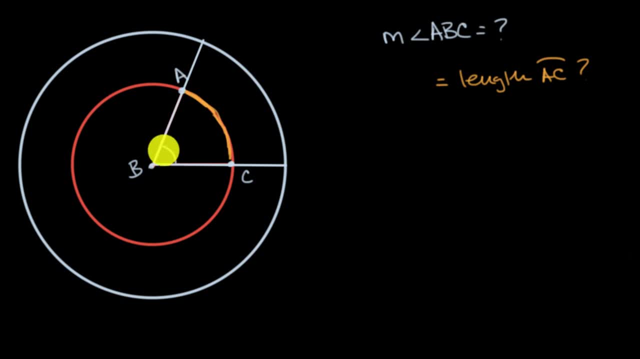 Let me introduce another circle here. So we have the same angle measure, the central angle, right over here. You could say angle ABC is still the same, but now it subtends a different arc in these two different circles. You have this arc right over here. 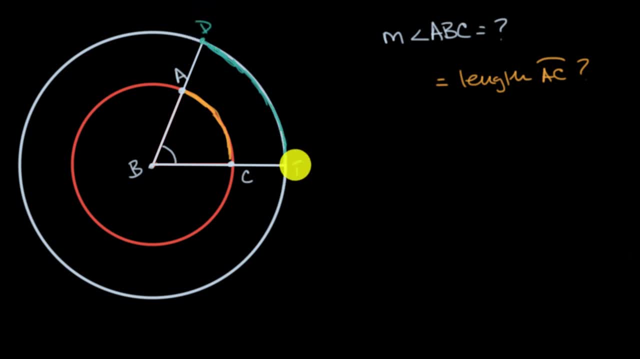 Let's call this arc DE, and the length of arc DE is not equal to the length of AC, And so we can't measure an angle just by the length of the arc that it subtends if that angle is a central angle in a circle. 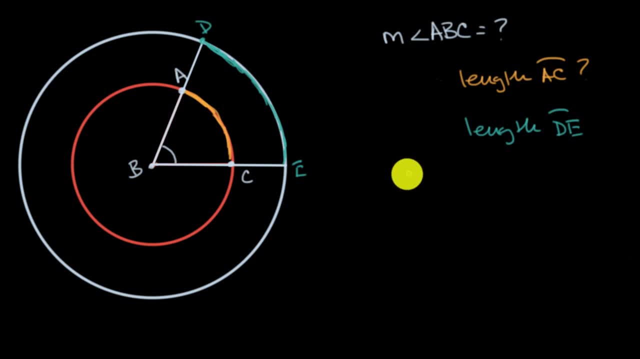 So we can get rid of that equality here. But what could we do? Well, you might realize that these two pi's that I just created, you could kind of say pi ABC and pi DBE, these are similar pi's. Now, we're not used to talking in terms of similar pi's. 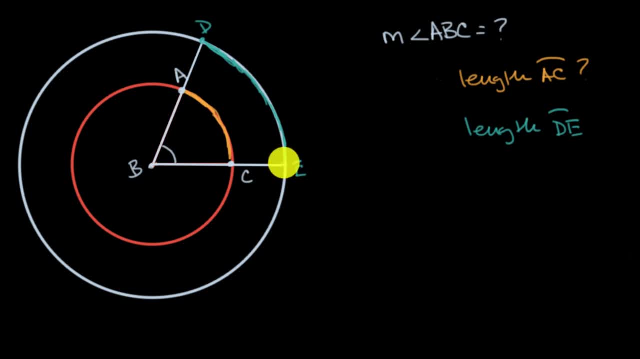 but what does it mean to be similar? Well, you have similarity if you can map one thing onto another, one shape onto another, through not just rigid transformations, but also through dilations. And in this situation, if you were to take pi ABC, 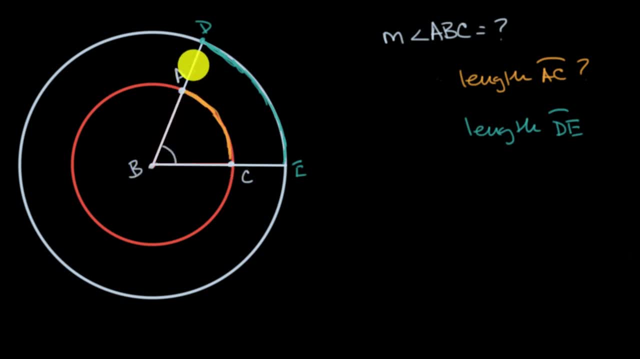 and just dilate it by a scale factor larger than one. there's some scale factor where you would dilate it out to pi, DBE, And what's interesting about that is if two things are similar, that means the ratio between corresponding parts are going to be the same. 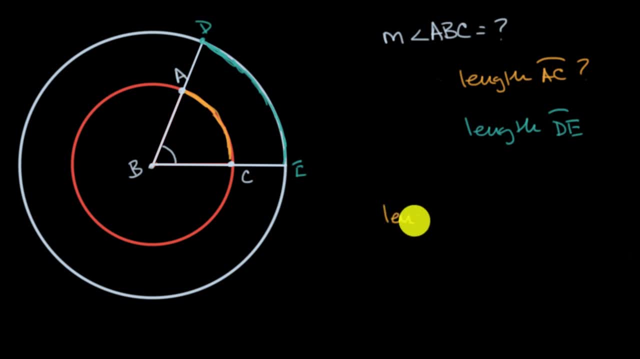 So, for example, the ratio of the length of arc AC to segment, the length of segment BC, is going to be equal to the ratio of the length of arc DE, DE to the length of segment BE. So maybe this is a good measure. 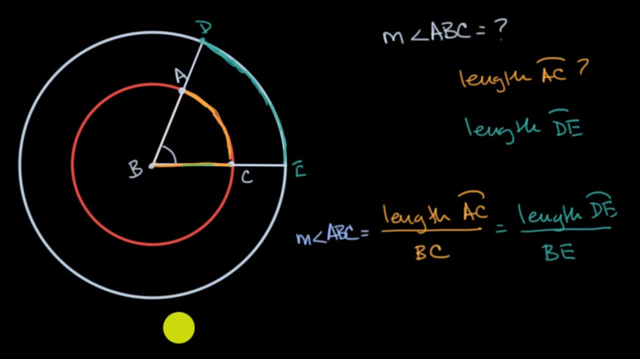 maybe this is a good measure for an angle, And it is indeed a measure that we use in geometry and trigonometry and throughout mathematics, And we call it the radian measure of an angle, of an angle, and it equals, equals the ratio. 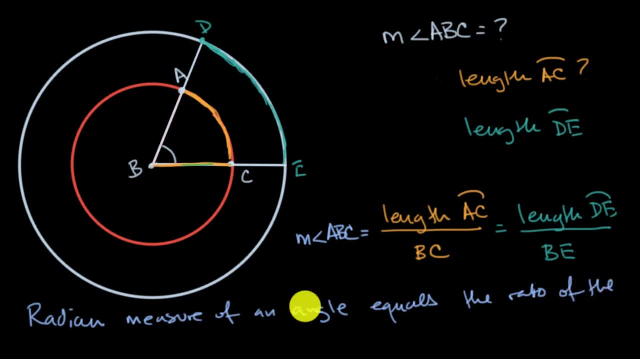 of the arc length subtended by that angle to the radius. We just saw that in both of these situations. So let's see if we can make this a little bit more tangible. Let's say, we had a circle here and it had a circle here. 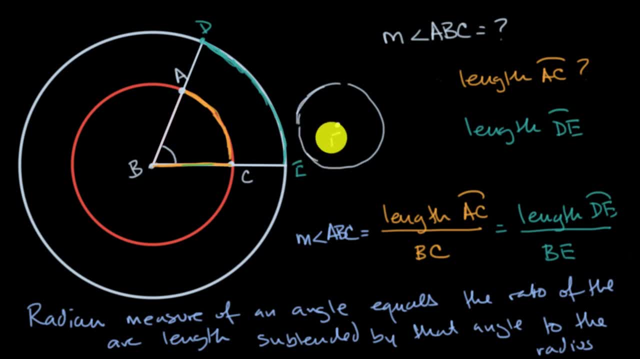 and it has a central point. Let's just call that point F, And then let me create an angle here, And actually I can make a right angle. So let's call it F and let's call this point G and let's call this H. 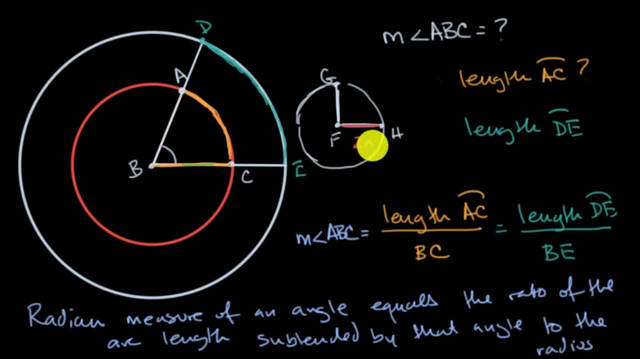 And let's say that the radius over here is two meters. And now, what would be the length of the arc subtended by angle GFH? Well, it's going to be one fourth the circumference of this entire circle, the way that I've drawn it. 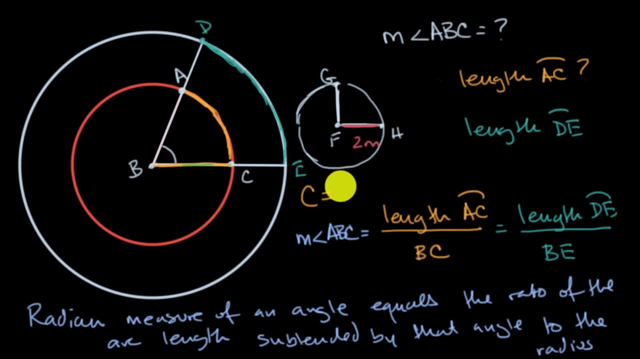 So the entire circumference- I could write it here- the circumference is going to be equal to two pi times the radius, which is going to be two pi times two meters is going to be four pi meters. And so if this arc length is one fourth of that,